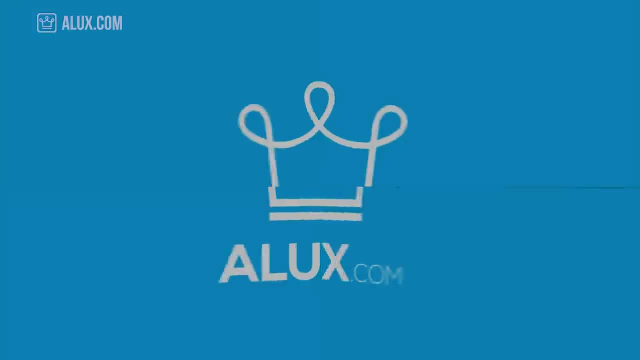 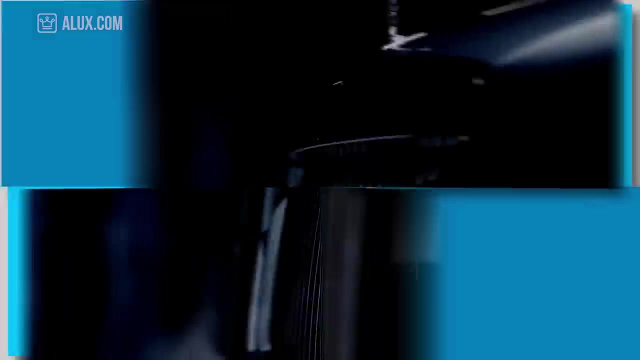 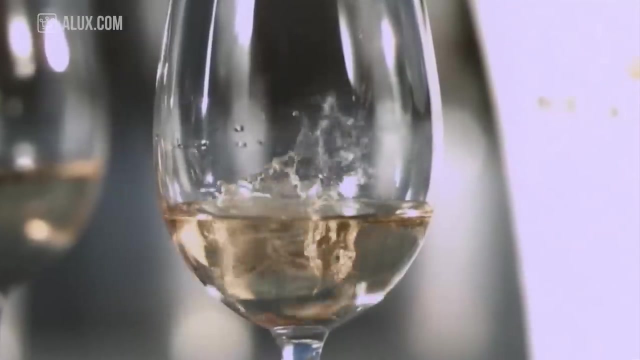 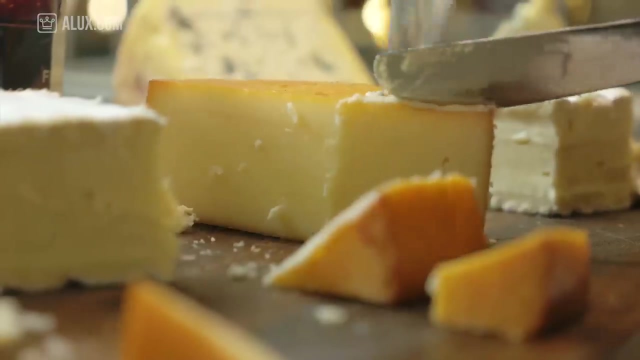 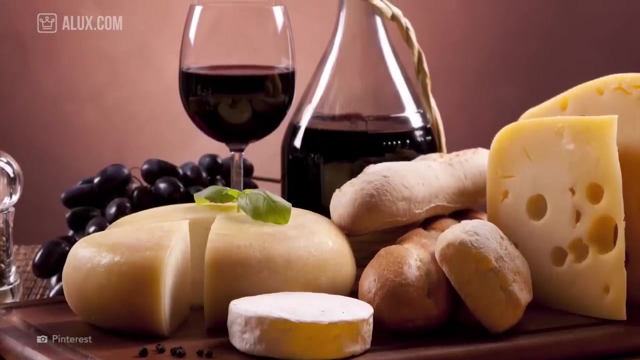 Welcome to ALUXcom, the place where future billionaires come to get inspired. Hello, Aluxers. today we're talking about the most exotic, tasty and, of course, most expensive cheeses in the world. Everyone is familiar with cheese. It's a common ingredient in most meals. 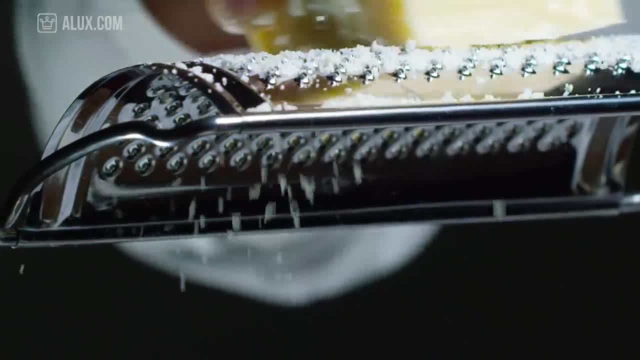 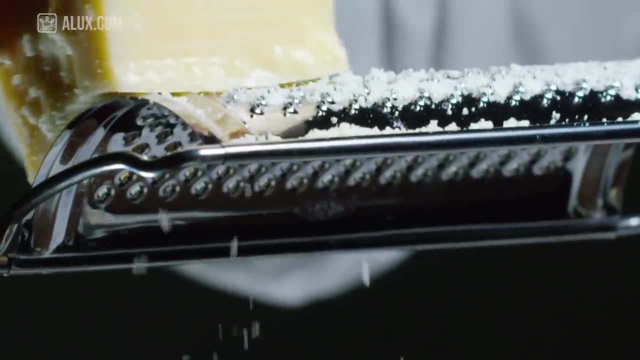 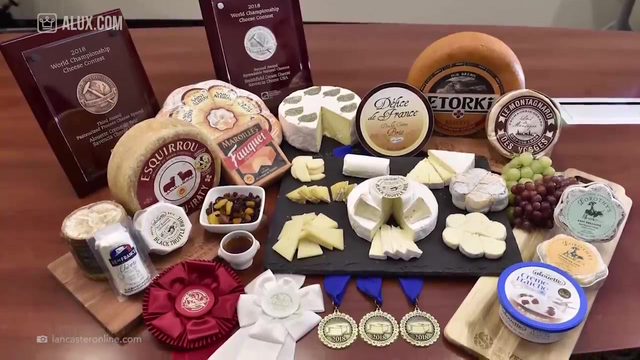 Everyone knows the common cheeses, such as American Provolone and Swiss, but there's an entire world out there of cheese that's judged on several traits, including taste, aroma and even aesthetic appearance. There are even gourmet cheese judges and competitions that rank cheeses by even more criteria. 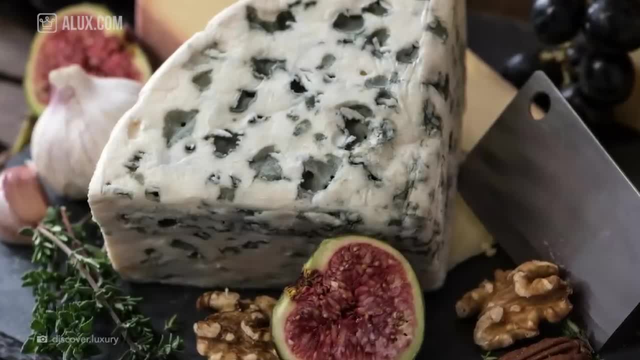 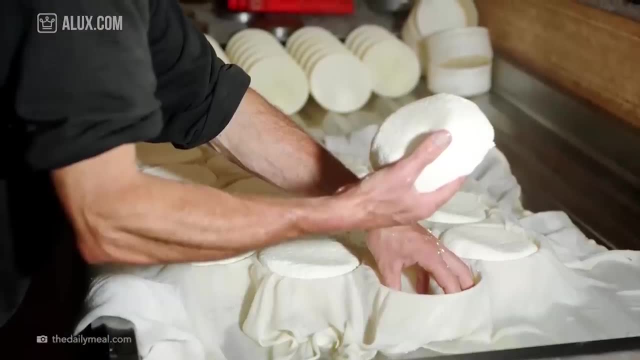 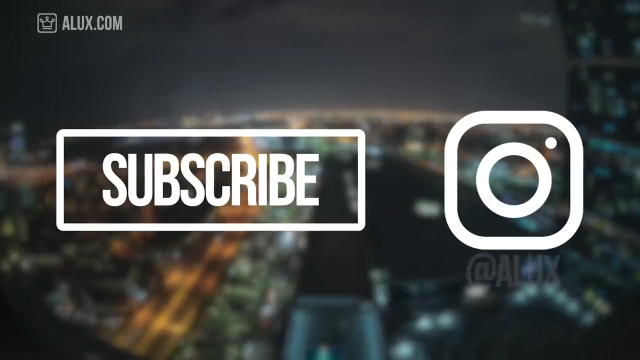 Although cheese is appreciated the world over, France perhaps will always remain the home of the best gourmet cheeses. So if you want to live the good life, it's time to start planning a trip. If you're new here, welcome. Be sure to subscribe and follow us on Instagram at ALUX. 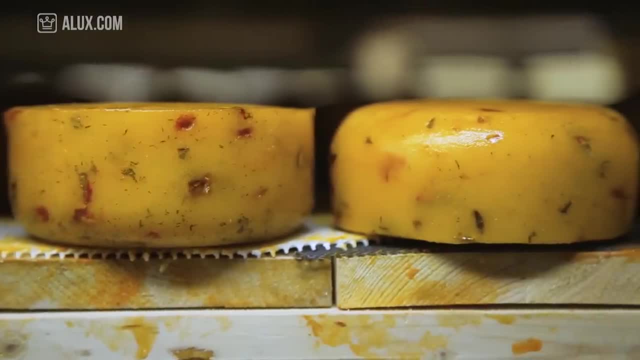 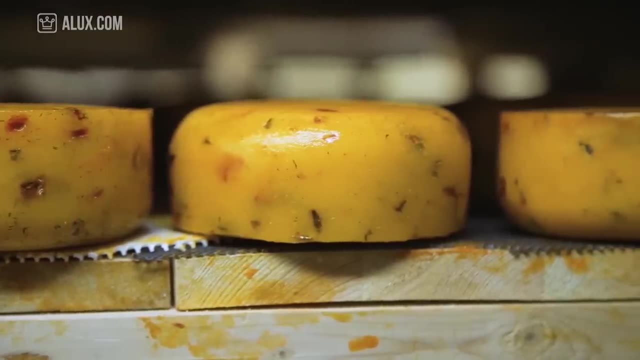 Now let's just dive in, shall we, and discover a bit of extravagance and the higher-end cheeses the world has to offer that many people will unfortunately miss out on. But hey, that's what you have us for And, as usual, we've got you covered. 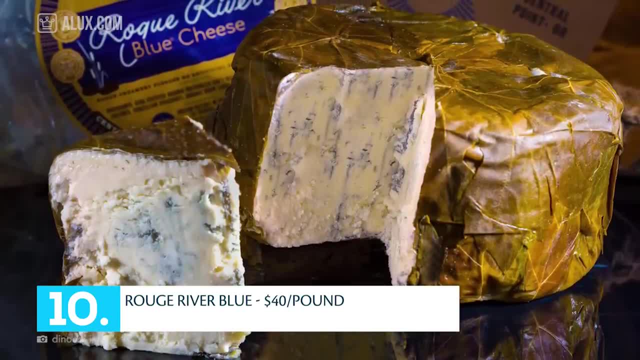 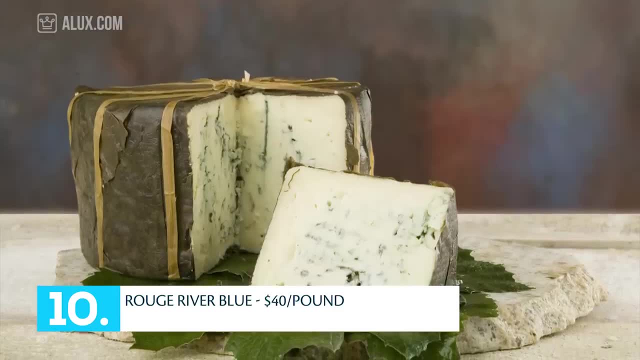 Rouge River Blue cheese is a seasonal cheese that can only be produced in summer, which is the one reason why it costs $40 for an eighth of a wheel. An interesting fact about the production of this cheese is that it's made with aged grape leaves soaked in pear brandy. This gives it a unique range of flavors that have been described as fruity, sour and sweet, and the most interesting of all the flavors can be the one that has the most protects the taste of every raw food. ROUGE RIVER BLUE CHEESE IS A SEASONAL CHEESE. This gives it a unique range of flavors that have been described as fruity and savory. ROUGE RIVER BLUE CHEESE IS A SEASONAL CHEESE THAT CAN ONLY BE PRODUCED IN SUMMER, which is the one reason why it's about 40 dollars for an eighth of a wheel. 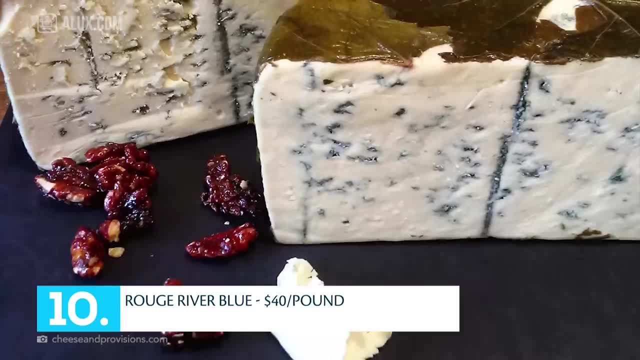 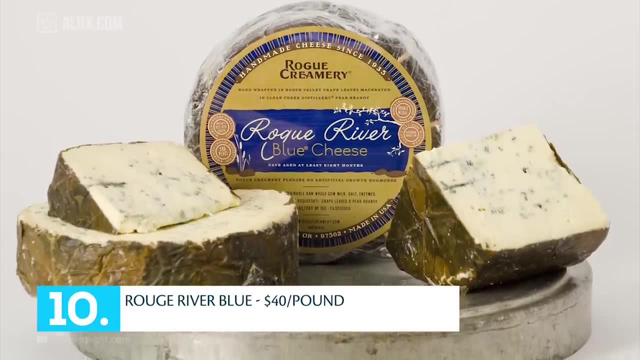 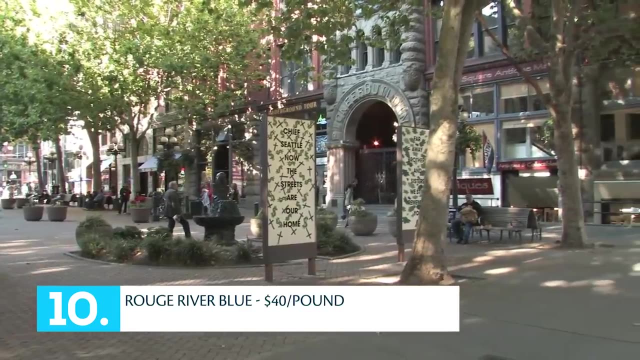 as fruity and spicy, with hints of hazelnut, blackberry, vanilla, chocolate and even bacon. The paste crystallizes with time, giving it more of a distinct quality. It will also be the single cheese on our list that's been produced originally in the US. in the state of Oregon, to be more precise, since 1930.. Although it's been around a long time, it's only recently gained worldwide acclaim when it won the 2003 World Cheese Awards in London. This Italian cheese offers a unique taste of the Mediterranean draw curd cheeses. 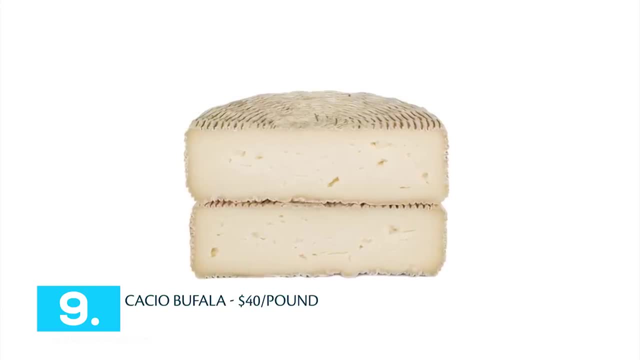 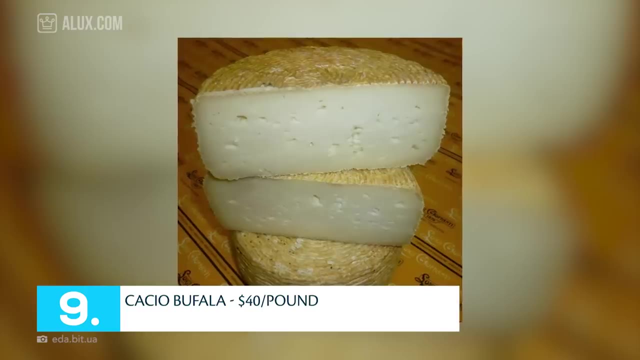 It's actually made using pasteurized water, buffalo milk. The curd is drained in such a manner it follows the natural maturing process. It's matured in the caves of the region for a period of up to a year. The result is a 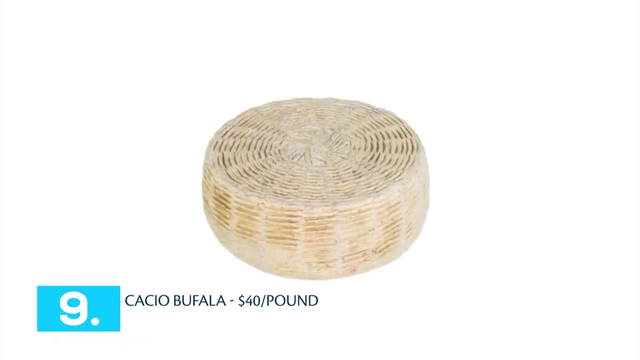 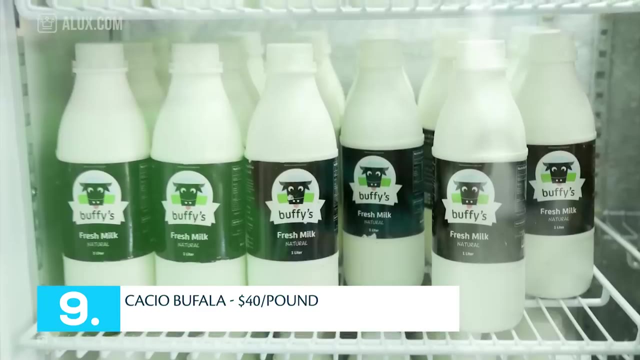 drum-shaped, ivory-yellow colored cheese, and it features the flavorful taste of buffalo milk. It's said that it literally melts in your mouth. This makes sense, as buffalo milk has twice the fat of cow's milk, so the result is a very creamy cheese. 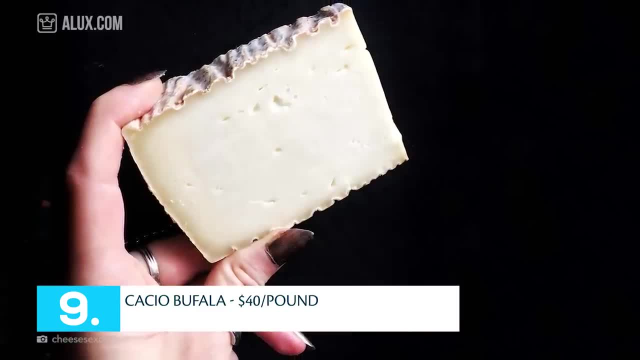 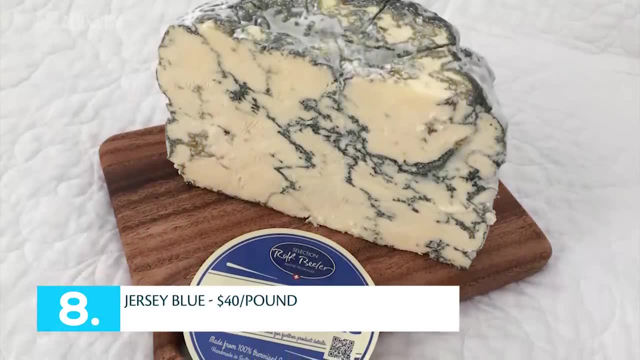 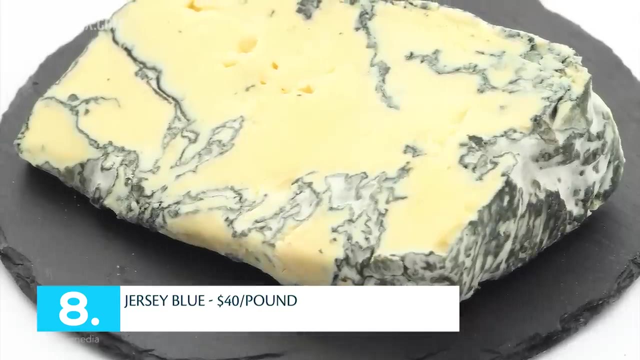 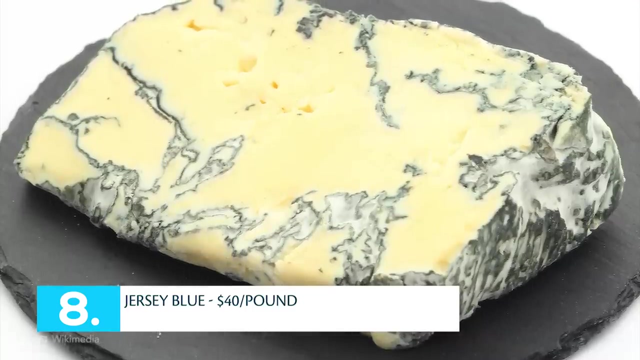 And with rare water buffalo milk as its main ingredient, it's no wonder this cheese comes in at $40 per pound. Another $40 a pound cheese. Jersey Blue Cheese is made from the raw milk of Jersey cows and formed into a whitish dome with blue veins running through it. 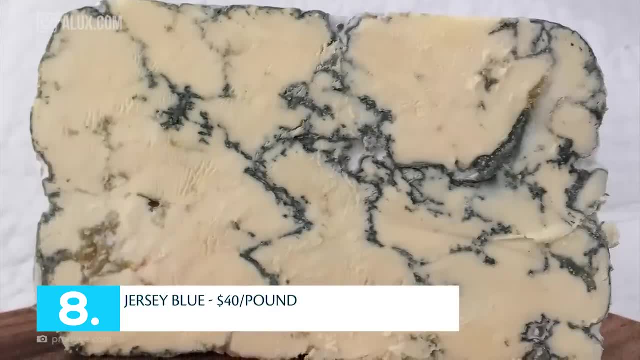 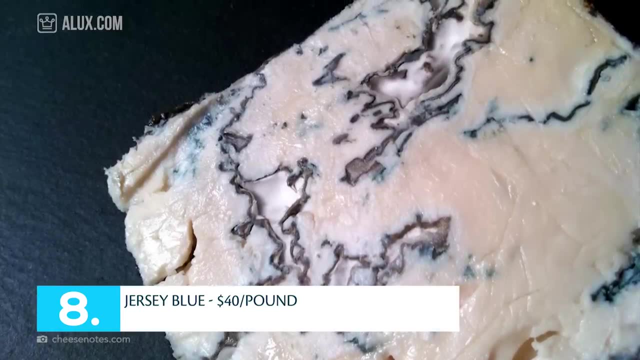 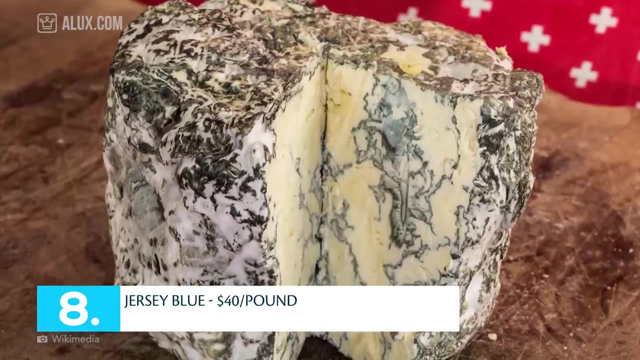 The cheese is made by hand and the veins are created by ladling the curds into a mold, which creates pockets. It gains a particularly musty aroma because it's aged in cold cellars. However, once it is cut, it produces a clean and even tangy scent. 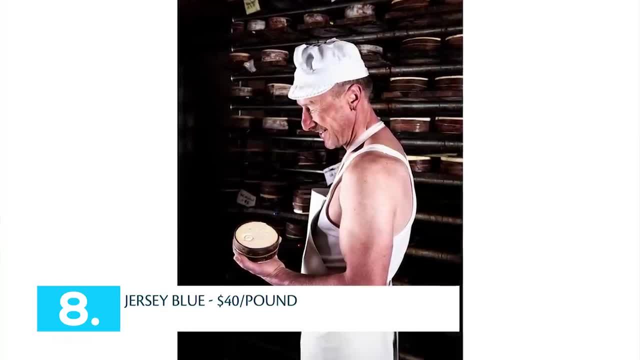 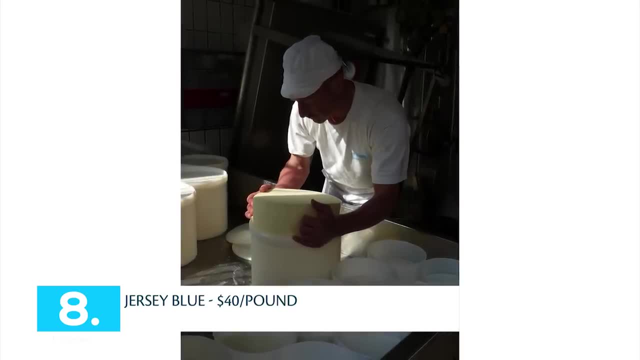 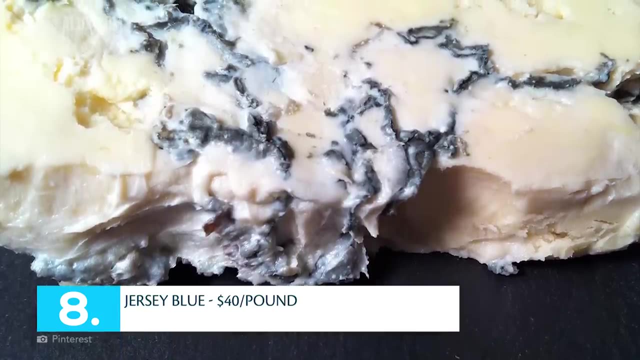 The cheese is a product of Will Schmid, who has run the dairy farm since 2006.. Schmid says he ages his cheese about 10 weeks, or sometimes longer if the blue veins have not yet formed. Although the cheese was originally produced in the UK, it's now manufactured in Switzerland. 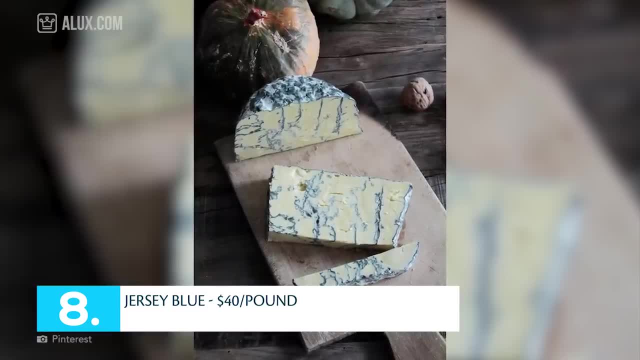 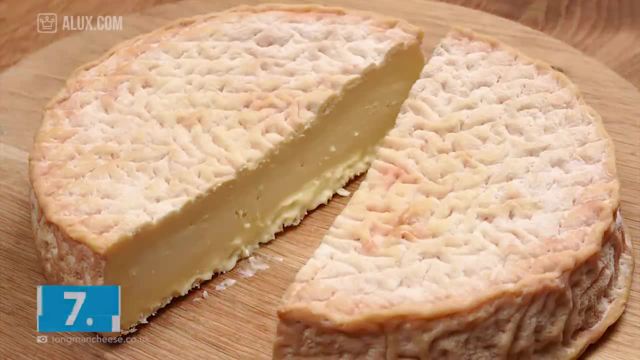 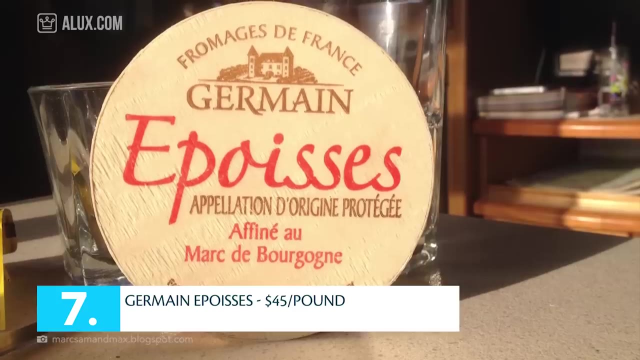 It can be eaten either new or aged. Fresh Jersey Blue is buttery, but when aged and dried out, its distinct flavors really pop. Number 7. Germain et Poissesse- $45 per pound. Germain et Poissesse is known for being one of the most pungent and runniest of cheeses, but it has a firm heart as well. 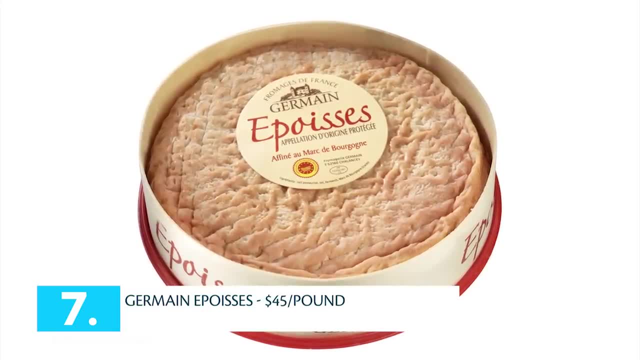 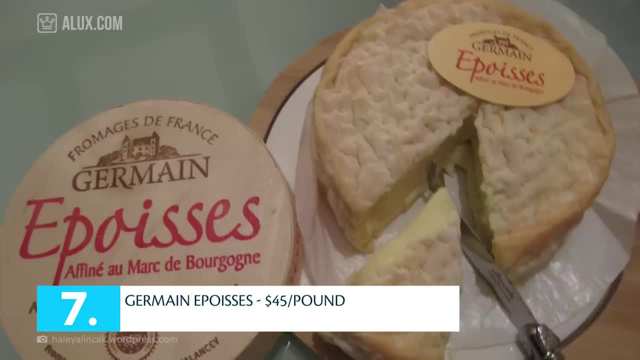 While other types of Poissesse have a strong scent and salty flavor, you'll find the Germain brand is a bit less salty and possesses more of a fruity flavor. It has a rather short aging period of only four weeks, where it's cured in humid cellars. 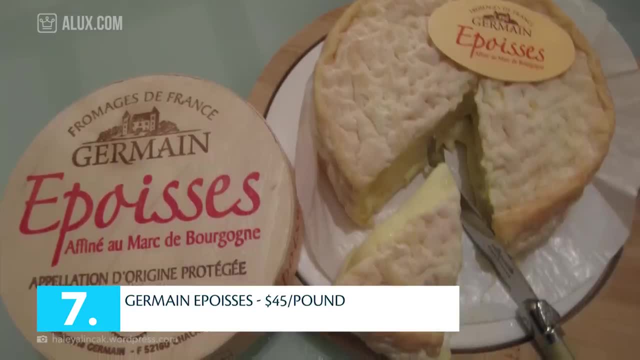 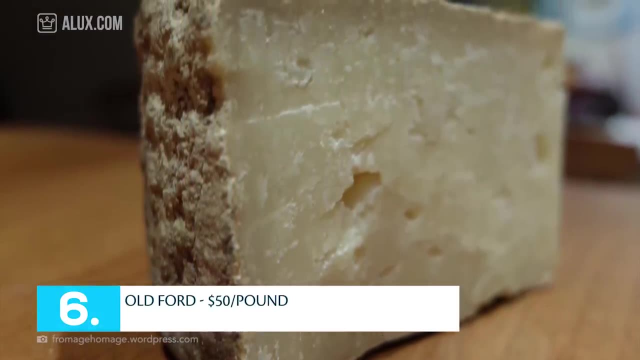 and then rinsed in Mark de Bourgogne to get good quality cheese Bourgogne, and it's available on the web for $45 a pound. Number 6. Old Ford – $50 per pound. Old Ford is a unique goat cheese that's aged to perfection. 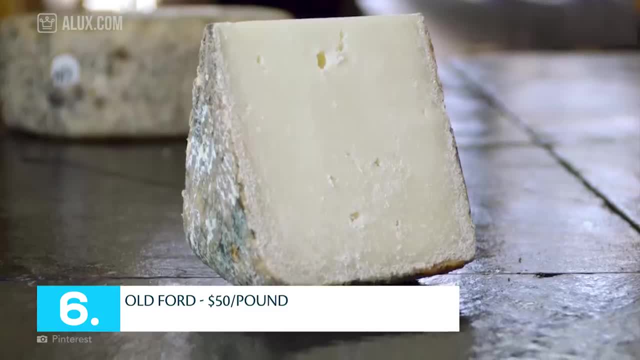 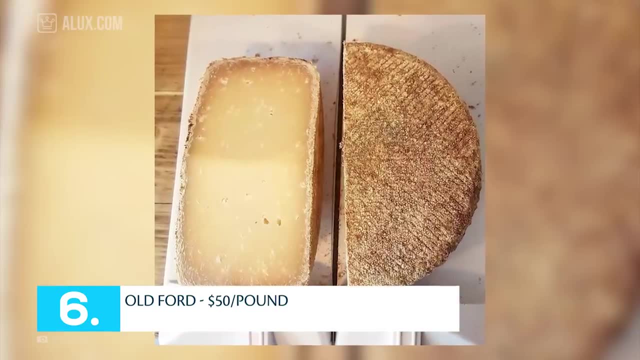 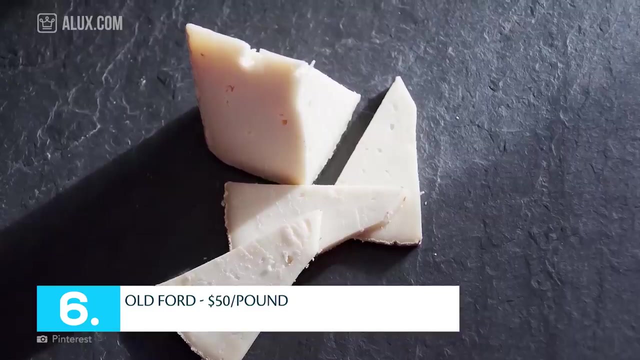 Usually because goats do not produce as much milk as cows. goat cheese is not aged very long, so this type breaks the mold a little bit by being a hand-pressed cheese that is aged. It's a laborious and time-consuming task, so, all things considered, the price tag is. 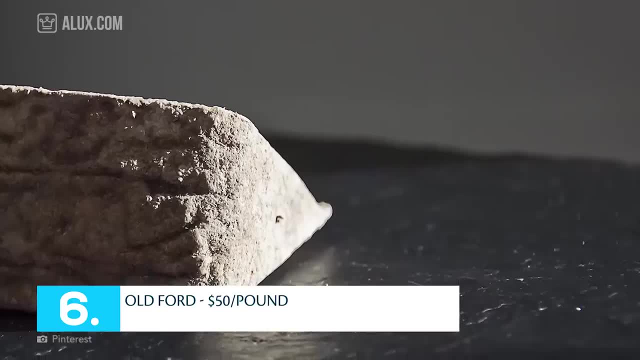 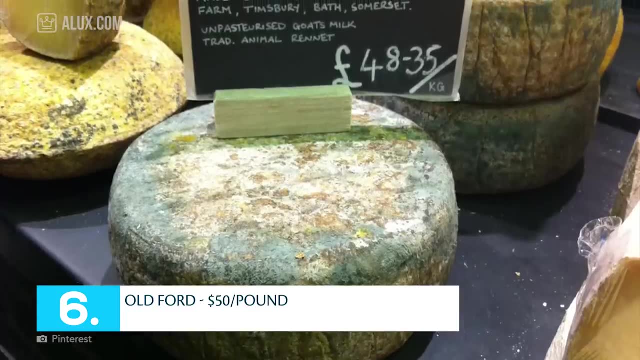 equal to the work that goes into it. It's best known for its unique taste that is described as earthy and floral. At $50 per pound it may be expensive, but not out of the question of the average person who wants to give it a try. 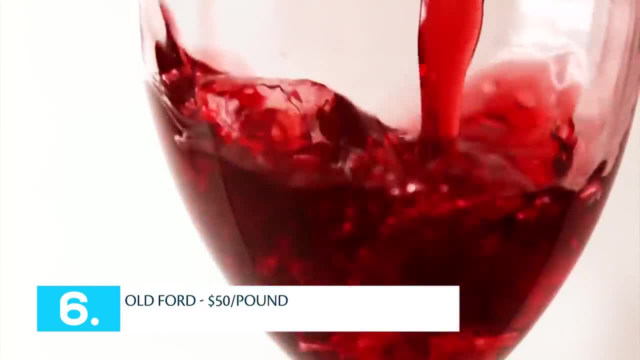 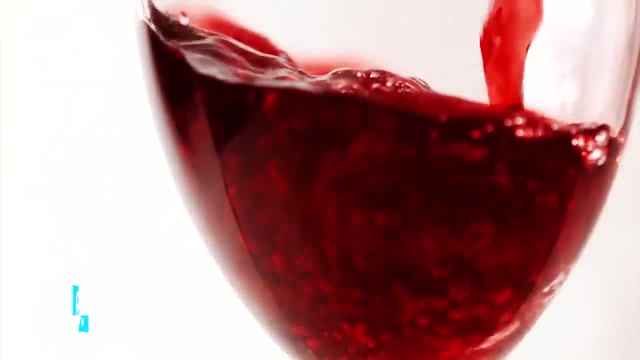 And if you want to pair a pricey wine with that cheese for the ultimate experience, click on the upper right-hand corner to check out our video. the 10 Most Expensive Wines in the World. Number 5. Cachucavalo, Puerto Rico – $50 per pound. 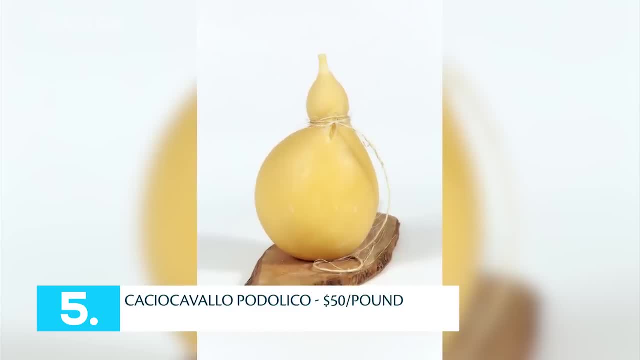 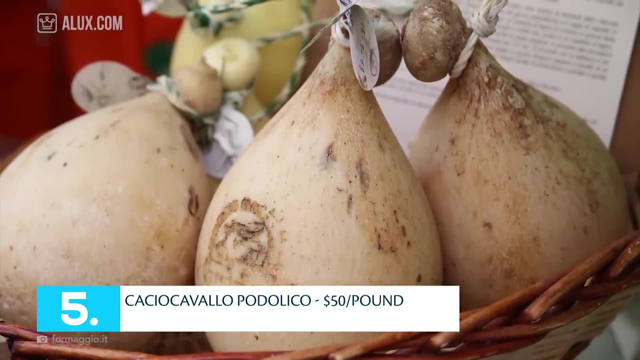 Although the name of Cachucavalo, Puerto Rico translates to horse cheese, it's in fact made of a very rare breed of cow, which makes it a candidate for one of the world's most expensive cheeses. While Cachucavalo is a fantastic cheese in itself, the strain that comes from the unique 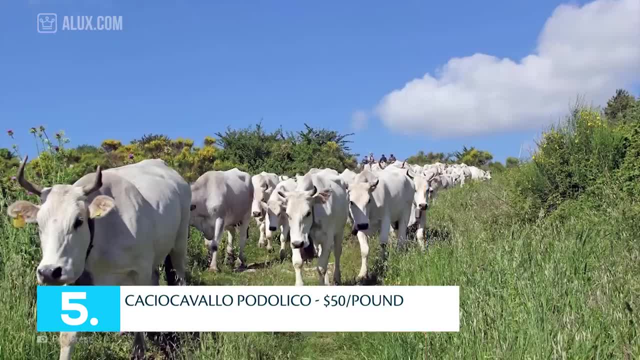 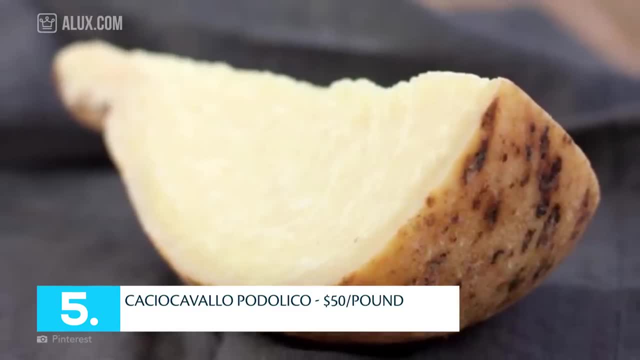 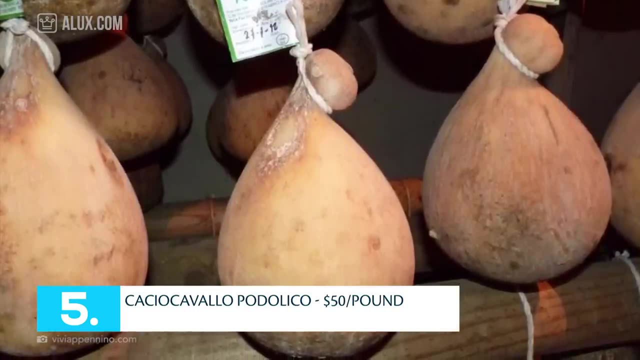 Puerto Rico variety is the most expensive. These cows don't produce very much milk. They produce very much milk due to the lack of water in their native region, which makes the cheese more difficult to find and, naturally, harder on the wallet. The region is, however, vital for the development of the cheese, as the cow's diet consists. 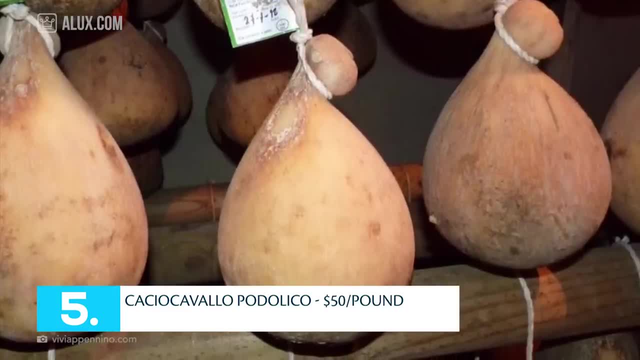 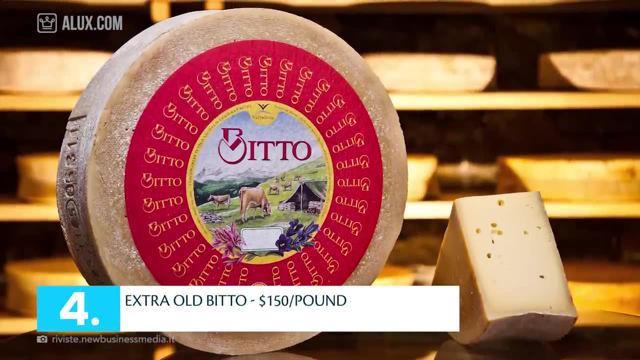 of licorice, fennel and myrtle, which has a strong influence on the taste of the cheese Number 4.. Extra Old Biddo – $150 per pound. China is known historically for many things, such as the fact that it is known for its unique taste. 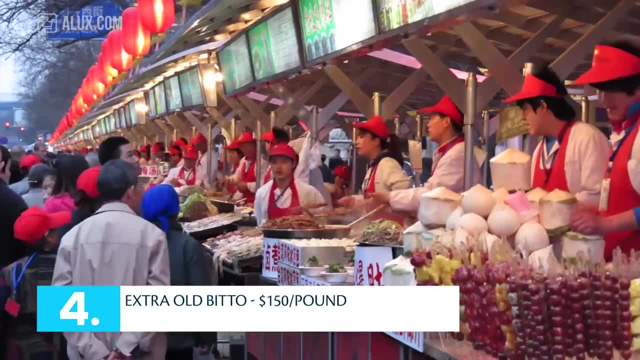 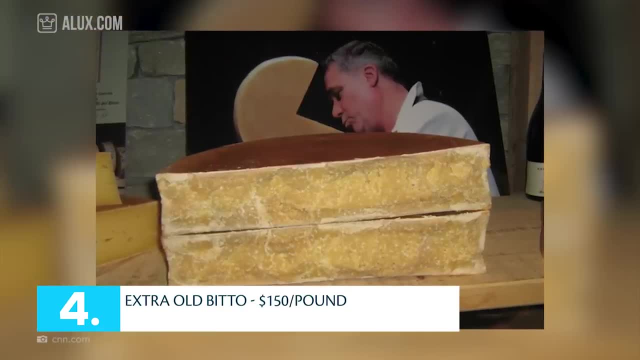 There are many things, but few people would think of it as being a producer of one of the world's most expensive cheeses. In fact, the 2,000-year-old recipe for Extra Old Biddo also makes it currently considered as the world's oldest type of cheese, with this batch being produced in 1997.. 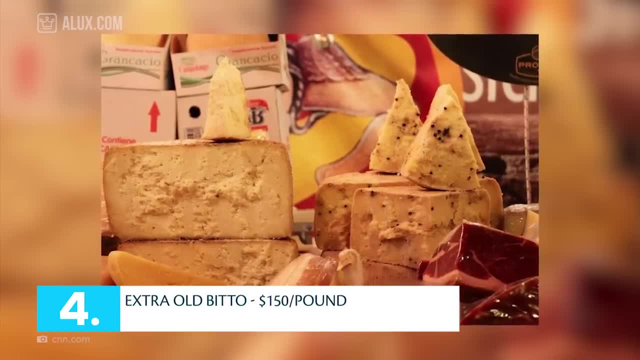 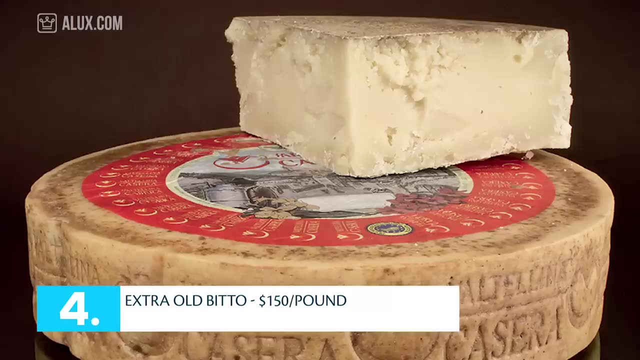 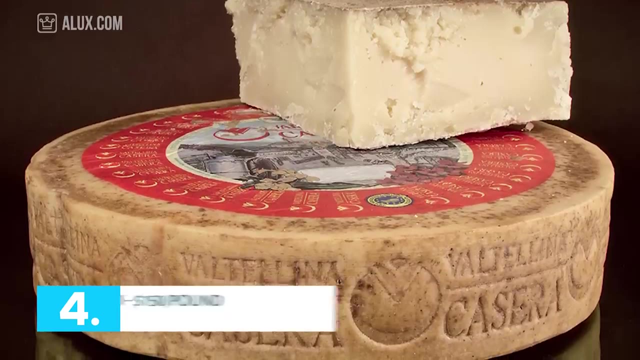 That's right. the oldest pieces of the cheese were produced 21 years ago and are currently found in China. It's supposedly only sold to Chinese citizens, but of course, all types of this cheese can be considered old, as it takes an amazing 10 years just for the cheese to mature. 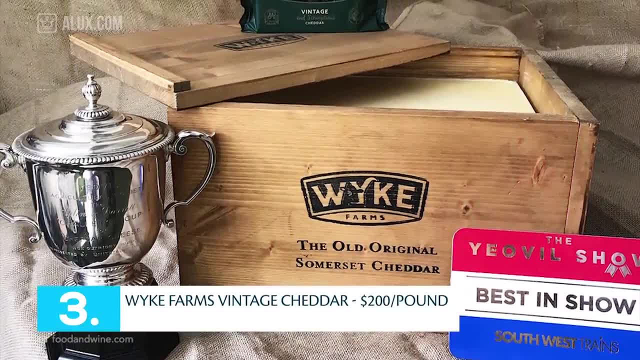 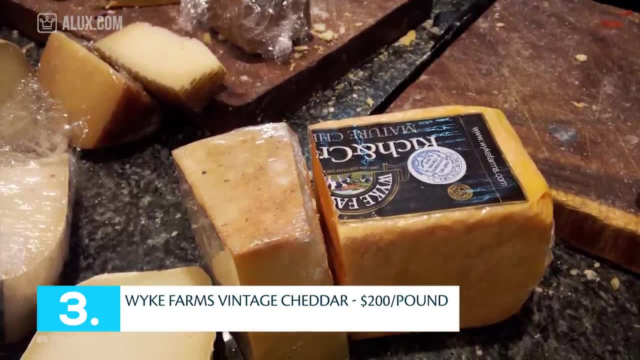 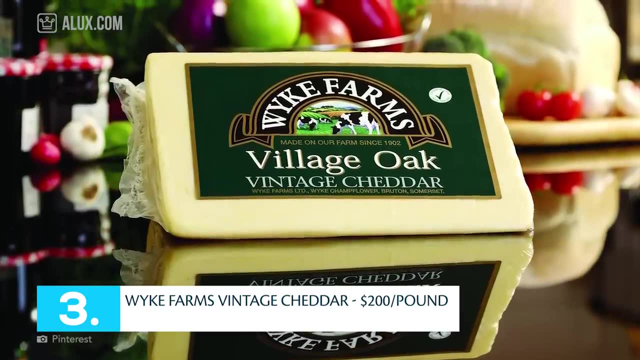 Number 3. Waikifarm's Vintage Cheddar – $200 per pound. With a price tag of $200 per pound, this is obviously not your average everyday cheddar you see at the supermarket. The Waikifarm's Vintage Cheddar is aged 15 months and is sold by the pound or sometimes. 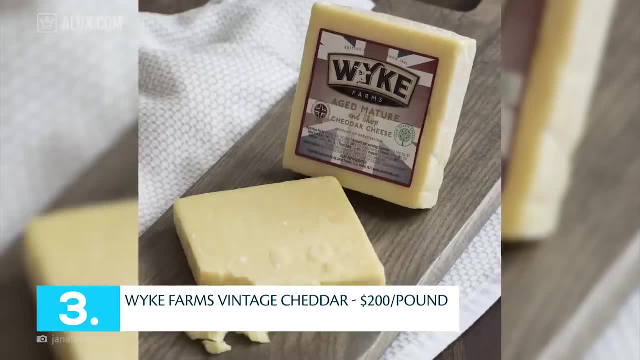 in other increments if you're a member of a certain club. The Waikifarm's Vintage Cheddar is sold by the pound or sometimes in other increments if you're a member of a certain club. It offers a unique and bold taste that is so charismatic of this unique blend of cheddar. 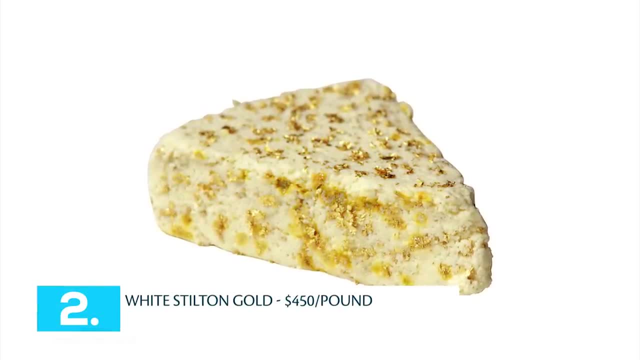 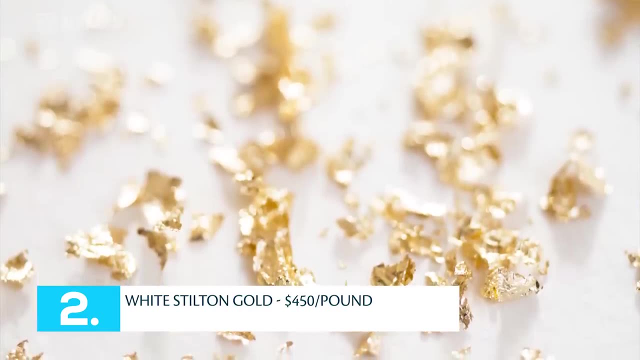 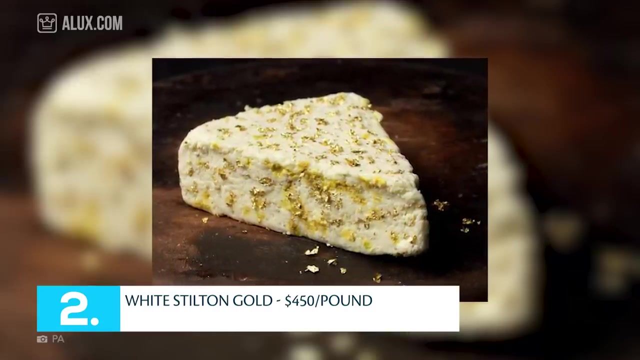 Number 2. White Stilton Gold – $450 per pound. You know, a cheese is elegant when it contains real specks of gold in it. White Stilton Gold cheese is $95 per slice and about $450 per pound. Think of this as an opulent version of the already pricey and rare Stilton cheese. 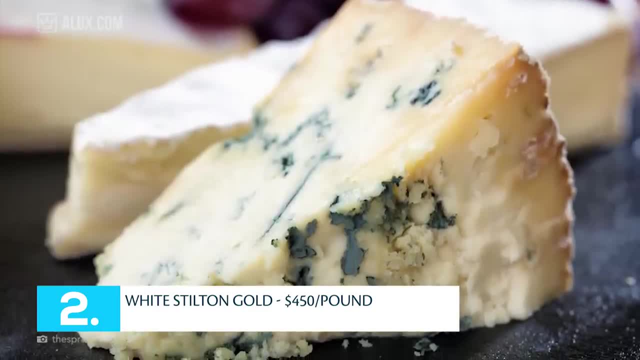 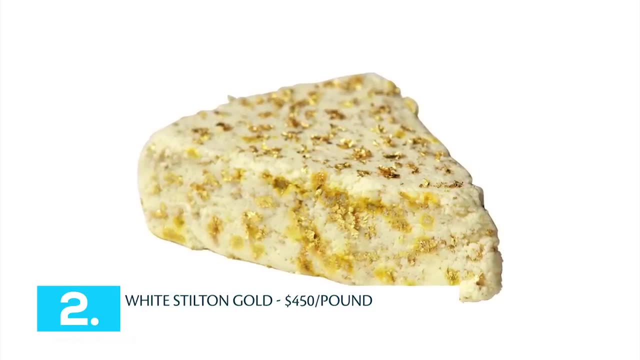 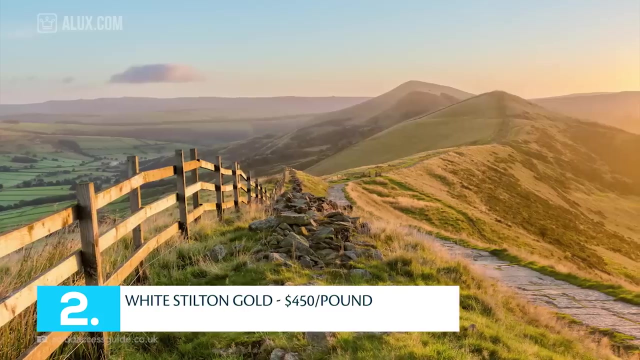 This is an English cheese historically, and it comes with both blue and white, both well known for their pungent smell and taste. What makes this cheese a rarity, besides the gold specks and all, is that it can only be produced by very strict standards in England. 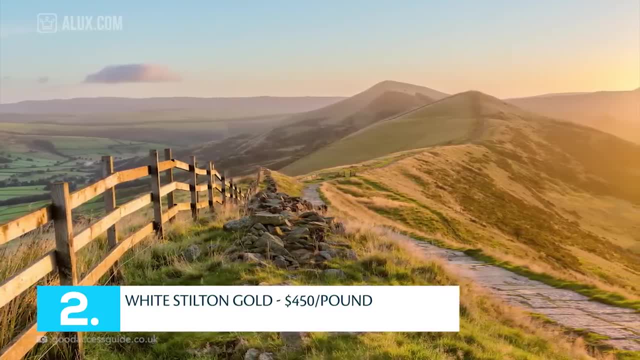 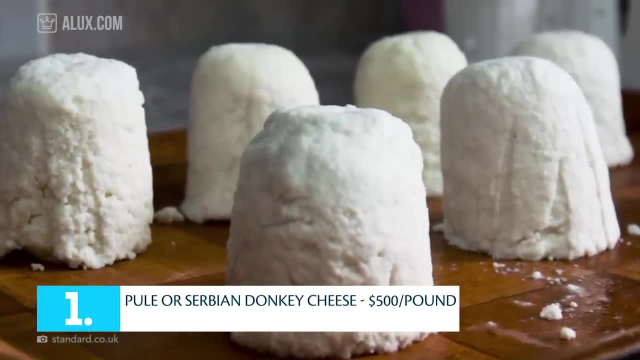 Actually make that. only 3 counties in England: Leicestershire, Derbyshire and Nottinghamshire. Number 1. Puel or Serbian Donkey Cheese – $500 per pound. This cheese is the best cheese in the world. It's the best cheese in the world. 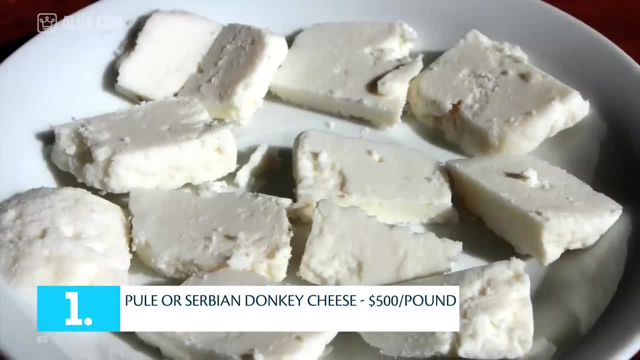 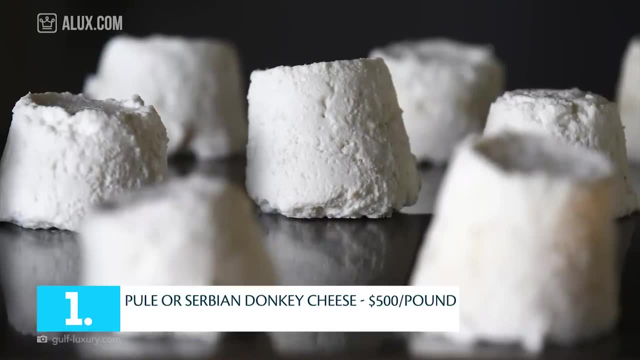 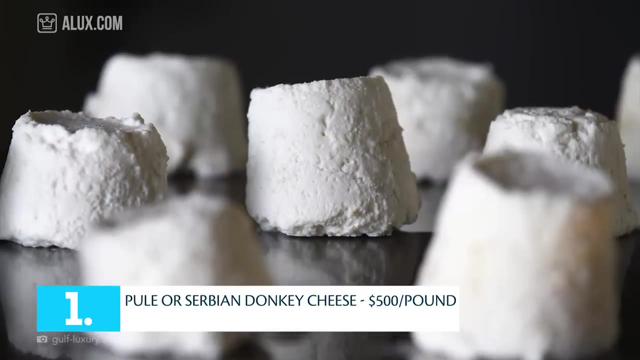 And here it is the most expensive cheese in the world. It's none other than Puel, or Serbian Donkey Cheese. Puel is also known in its native Serbian tongue as Magareci, and is the world's rarest and most expensive cheese, with an average price of around $500 per pound. 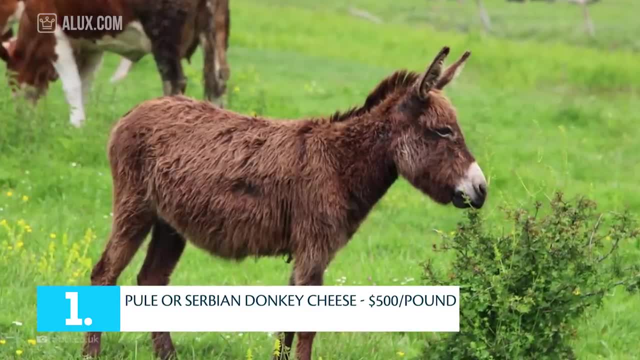 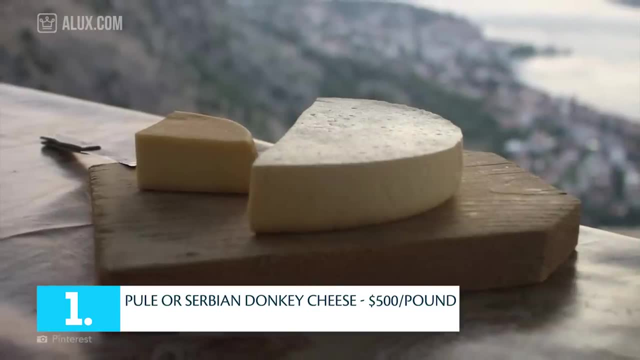 It's also known as Serbian Donkey Cheese, and, yes, this cheese is actually made from donkey milk. This is one of the many reasons why it's such an expensive cheese. It takes 25 liters of donkey milk just to make 1 kilo of the cheese, and it can only 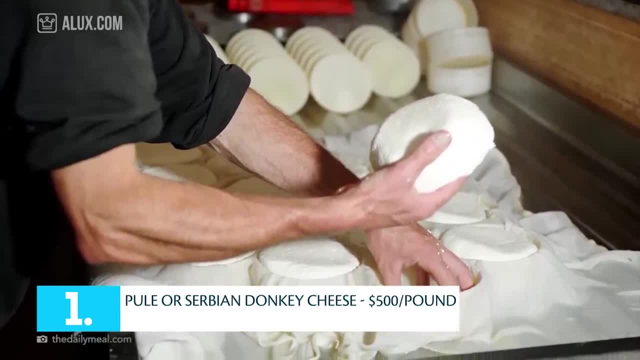 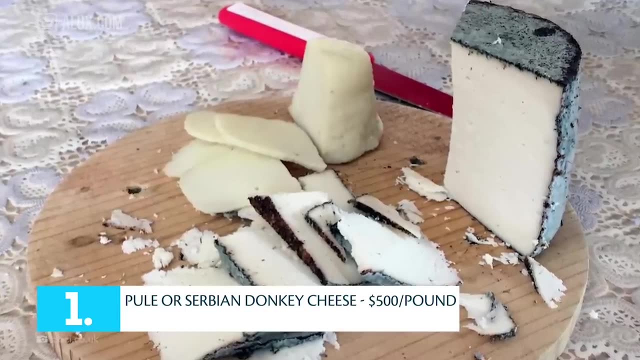 be authentically crafted by expert cheesemakers in Serbia, who've been producing this product for centuries. While 60% of the cheese is made with donkey milk, the remaining 40% is actually produced by goats, so it makes for an interesting mix. 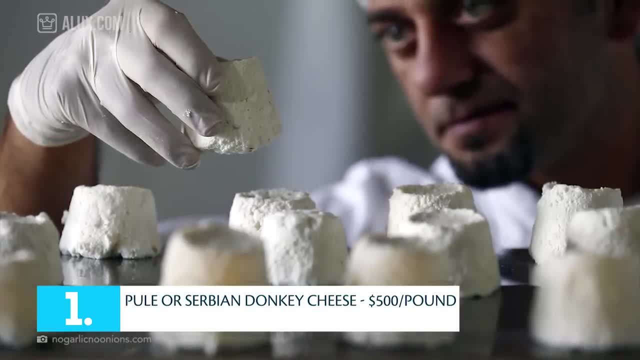 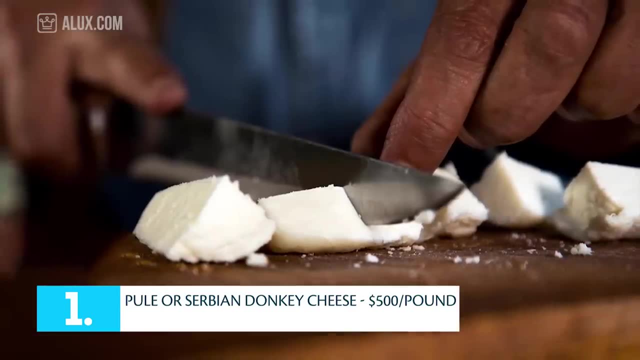 It's typically produced in cupcake-sized pieces, which makes it more affordable. This is a crumbly delicacy and you owe it to yourself to try it at least once, if only so you can tell people that you've eaten the most expensive cheese in the world. 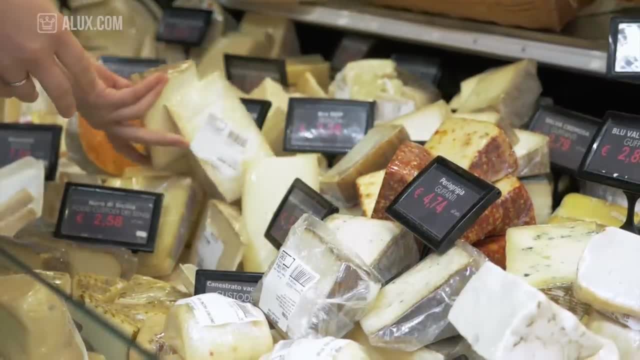 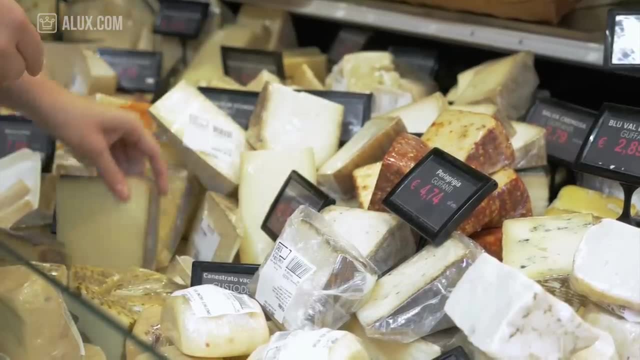 And that's it for today. Aluxers the top 10 most expensive cheeses in the world. But don't judge a cheese based on its cost alone. Take the time to actually enjoy the cheeses and other foods when you're at a higher-end restaurant or grocery store, so you too can. 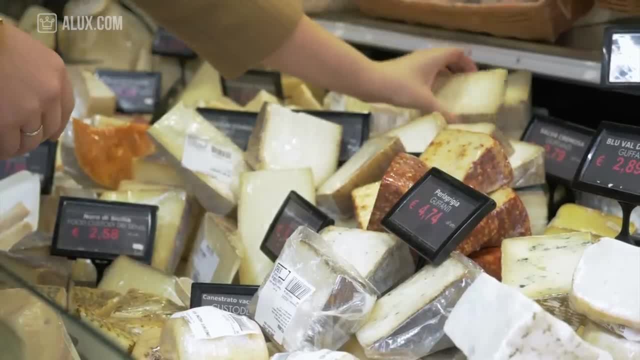 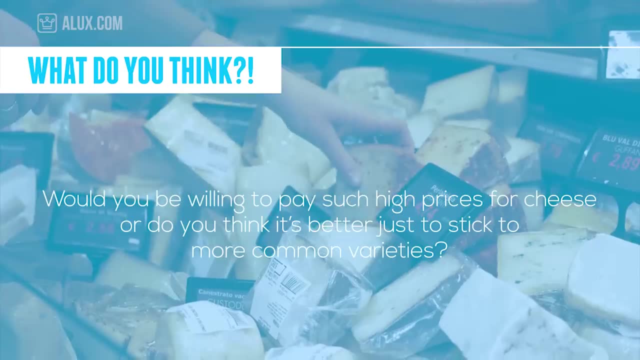 be a cheese judge and aficionado, And now that we've worked our way through this list, we'd like to know… Would you be willing to pay such a high price for cheese, or do you think that money would be better spent on something else? Let us know in the comments. 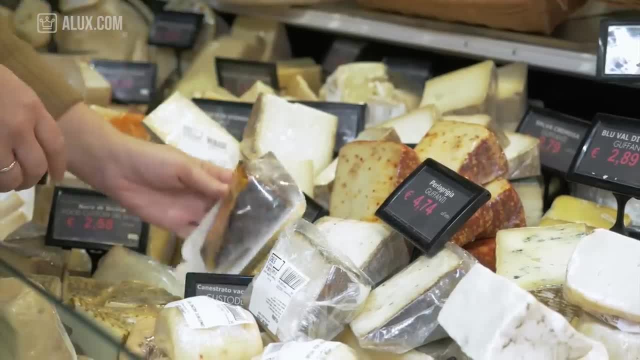 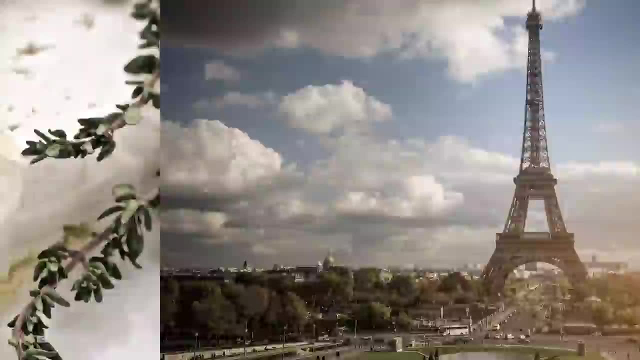 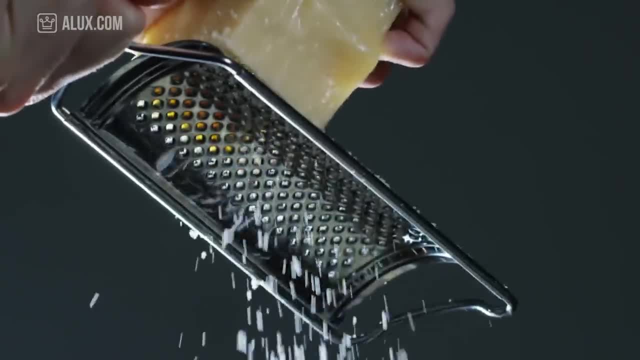 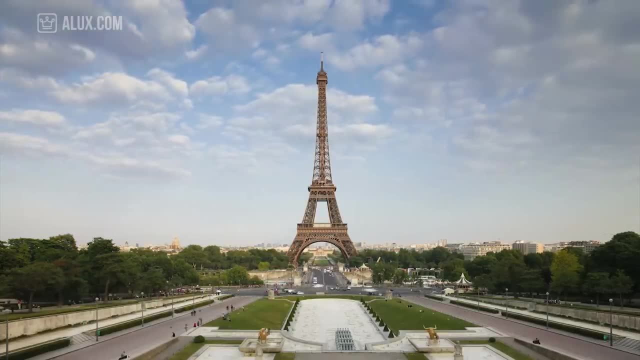 France may be the most well-known for their cheeses, and the United States produces the most cheese out of any country, but it's actually the people of Greece who claim the top spot for cheese consumption every year. France exports over 2.5 billion dollars in cheese products every year. and one can only imagine that a large portion of that goes to the Greek people, who each eat an average of 68.5 pounds of cheese every year. Thank you for spending some time with us, Aluxer. Make sure to subscribe so you never miss a video.